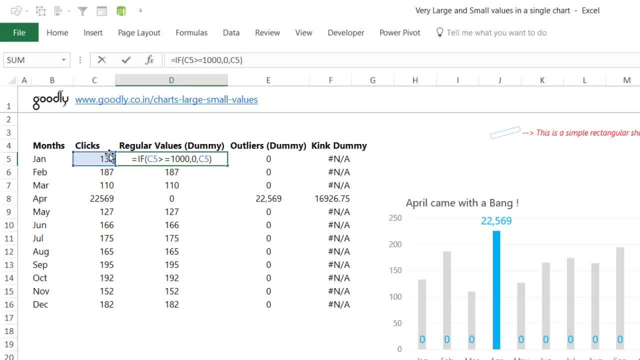 one is for outliers. Let's just take a look at a small formula. So I'm just saying that if this value is greater than a thousand, thousand is a benchmark which defines that. is this value considered a dummy or not? So if the value is more than thousand, then give me a zero. 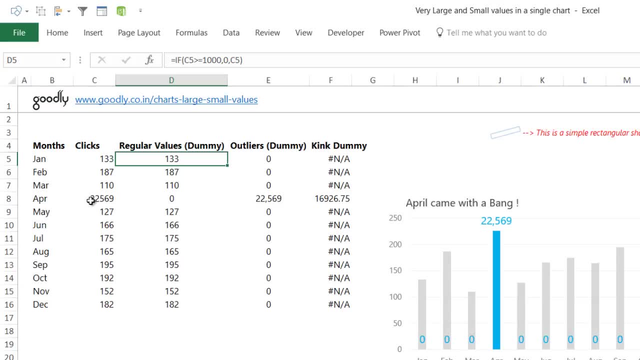 otherwise give me the same value and I drag the formulas down. So here the value was definitely more than thousand and that's the reason why you got a zero. Then the next outlier is for the outlier dummy. Sorry, the next dummy is for the outlier. So I'm saying the reverse logic. If 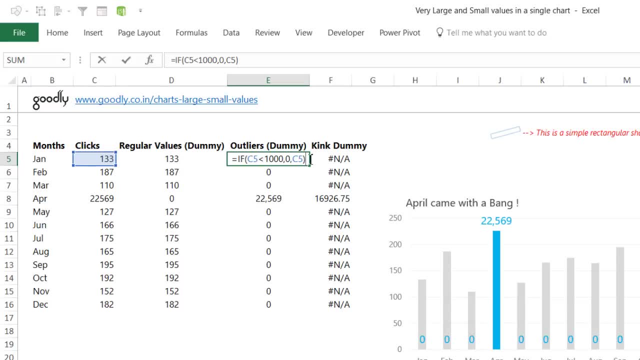 this value is less than a thousand, then give me a zero, otherwise give me the same value. So, since this value is definitely not less than thousand, it's more than thousand. So you're getting the value right here. So we create two dummies. The first dummy is this one, the second dummy is this one. 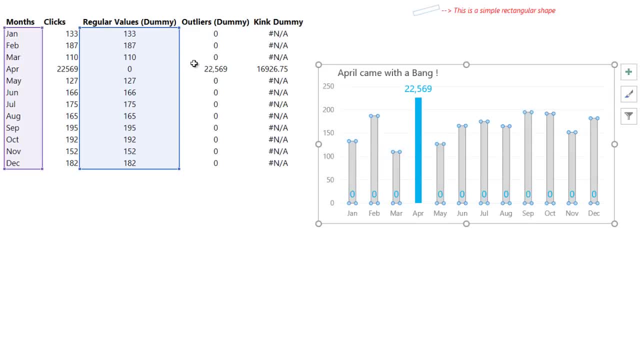 and that's what we do. So we place the gray bars on the primary axis with those regular values, and the other one- sorry, and this one is the outliers dummy- that we place it on the secondary axis. That's what we do And we get a chart like that. If you just take a look at the chart, I'm just 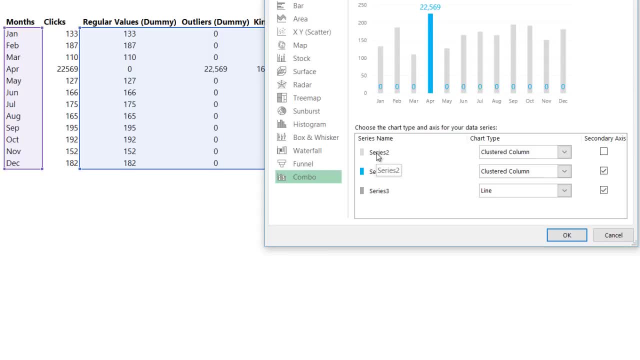 going to go and change chart type. You can just take a look that series two, which is my regular values, are on the primary axis and series one, which is my outliers, is on the secondary axis. So once we have a chart like this, we can have data labels and we can 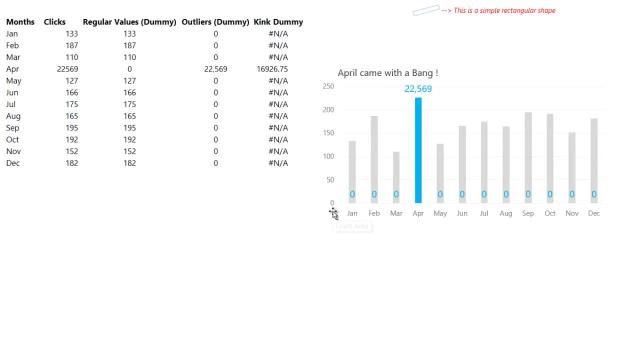 clearly see that this value stands out. But if somebody starts to read this chart, this is definitely not going to make sense because the chart is not broken. You have the axis up till 250 and you are showing 22,000 here, So we need to kind of break the chart with a kink. 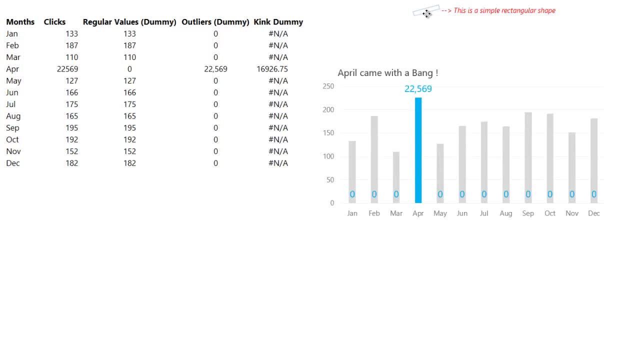 The kink is nothing but like a shape. Let's say, this is one shape that I've made. It can be here. it can be here, sorry, it can be here. it can be here. it can be wherever in the chart. So 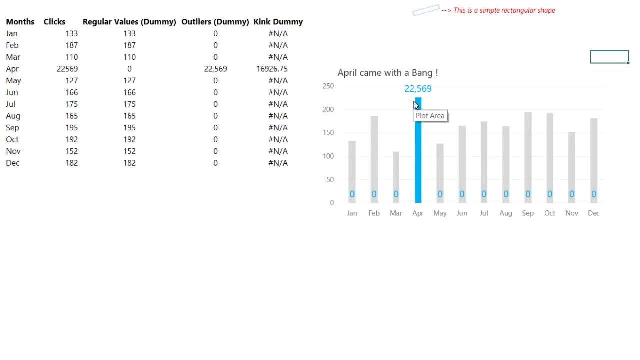 to decide where the kink is going to be. I have thought that the kink is going to be on the 75th percentage of the value. So if this is 22,000, I take 75% of that Somewhere. here is going to. 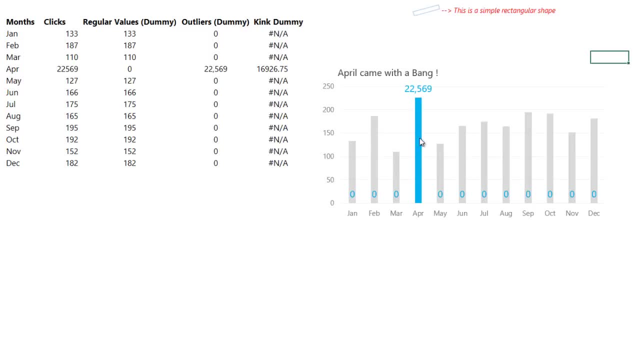 be the kink. You can decide wherever you want the kink: somewhere on the top, somewhere here, somewhere here, wherever you would like to have, You can have the kink. Kink is nothing but like a broken sign. So here's another dummy for kink. 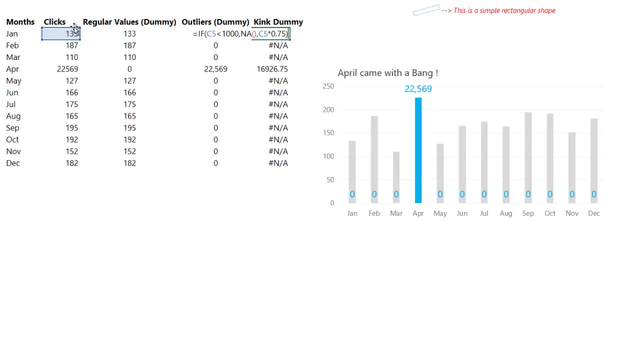 I say that. the same logic. if this value is less than a thousand, then take this value and multiply it with 75%. Otherwise give me an. any, That's what I say, And I drag it down. So as soon as. 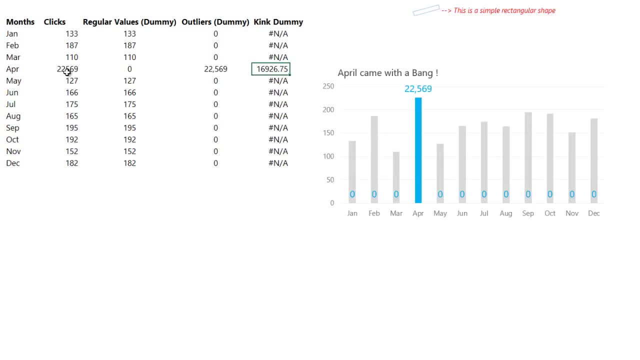 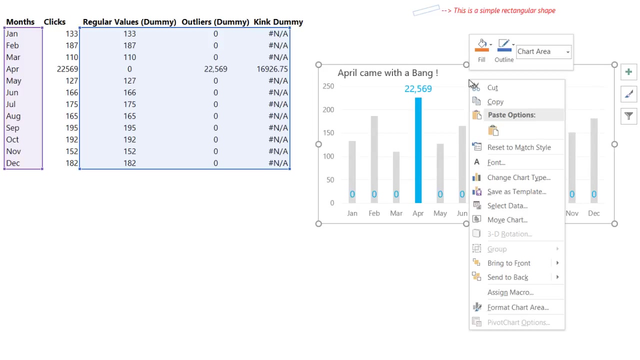 the Excel. if formula comes here, it finds the value is more than 22,000. It multiplies that with 0.75 and you get a value like here Again, I'm just going to do and put it in the chart And so let me just do that actually. So I'm just going to say: 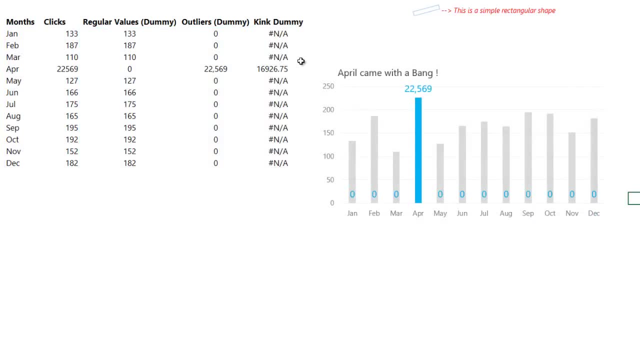 just delete that. Series 3 is nothing but the kink. I'm just going to delete that and do it once again. So here is the kink. So I'm just going to say Ctrl C to copy the data pick up. 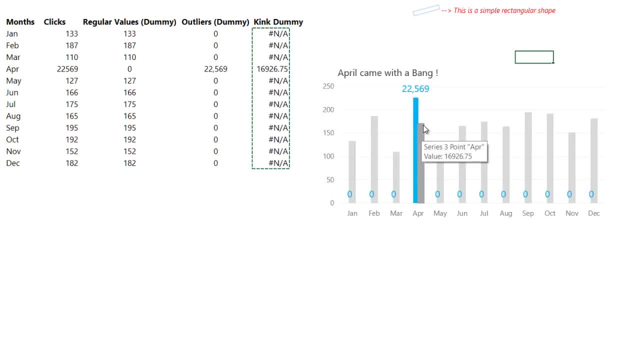 the chart: Ctrl V to paste the chart on the chart. And I have the kink right here. Now I'm just going to say, hey, right, click here, and then change the chart type, And I'm just going to say that instead. 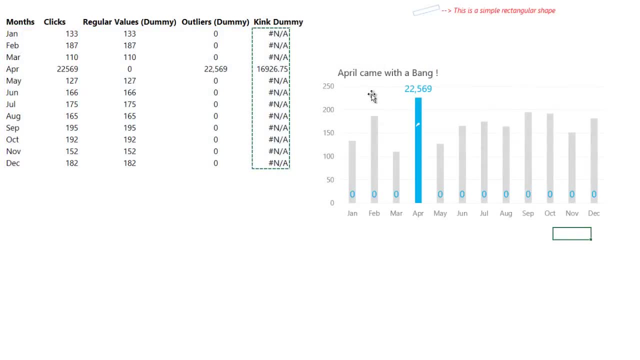 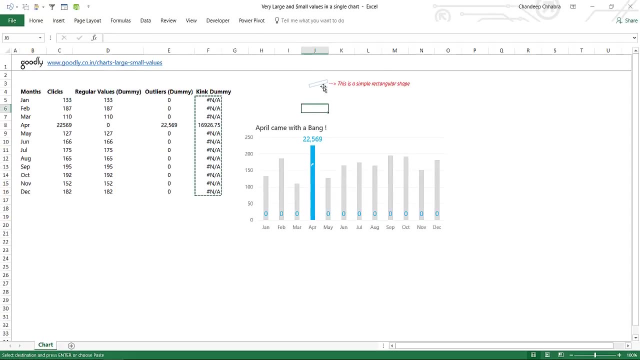 of a line chart with markers and I'm just going to say okay, And you get a kink, a small dot here or whatever here. Now what you can do is make a shape. So this is nothing but a shape. So I went. 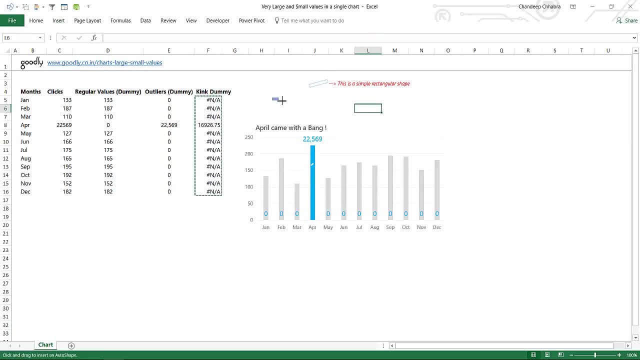 to the insert tab. I went to the shapes and I made a little rectangle like this and filled it with white color and outline was like a light blue or something, something like this, And I just tilted it a little to the left-hand side. That's all is the kink. 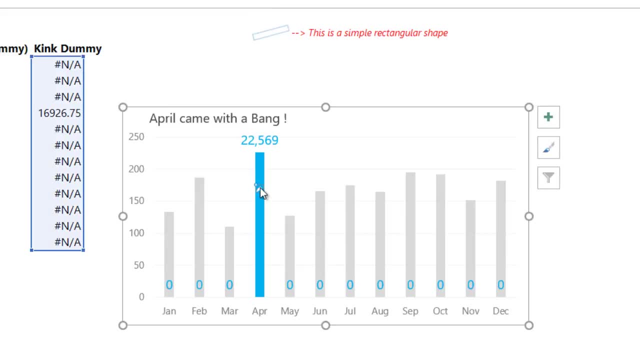 And then, once I made the shape, I'm just going to copy the shape and pick up that marker and say Ctrl V on that. So Ctrl C and then Ctrl V right here and you get a kink. Now the only problem with this chart is that you have a couple of zeros here, which you definitely don't want to see. So 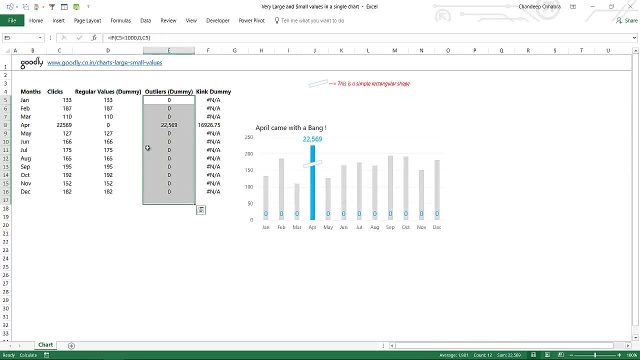 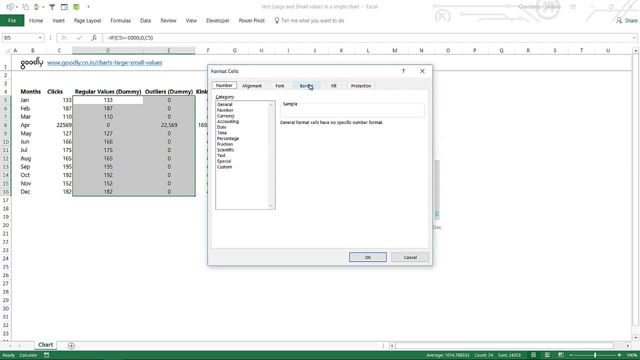 the zeros are coming from here. You can see that you have a zero here and a ton of zeros here, So what you can do is custom format this. I'm going to pick up these two columns, press Ctrl 1 to format this And I'm going to go in.